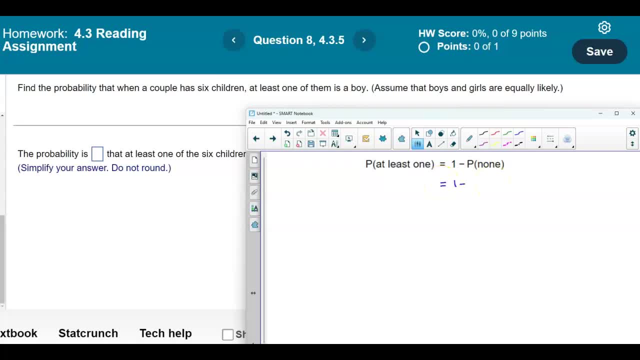 So that would mean that we're looking for one, minus the probability that all of them are girls. Ok, now, how many children are they saying that the couple is having? Well, that means that there's six of them. So if there's six of them, then that means that. 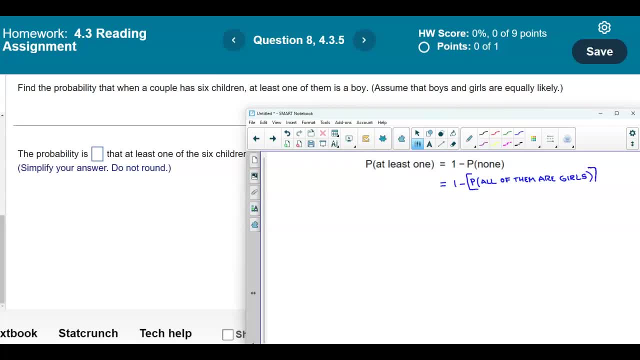 we're taking this probability and then we're going to multiply it six times, So we're going to raise this to the sixth power. Now what is the probability of getting one girl? Well, the probability of getting one girl is one out of two. So this would be one minus one over two. 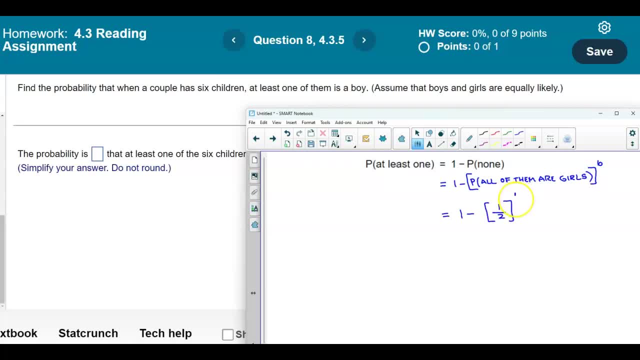 to the sixth power, since we're multiplying that six times, because that means that six of those children will be one out of two that are all girls. So now we need to simplify this. So we're going to take one, and now, if we take one and then raise it to the sixth power, that's going to give? 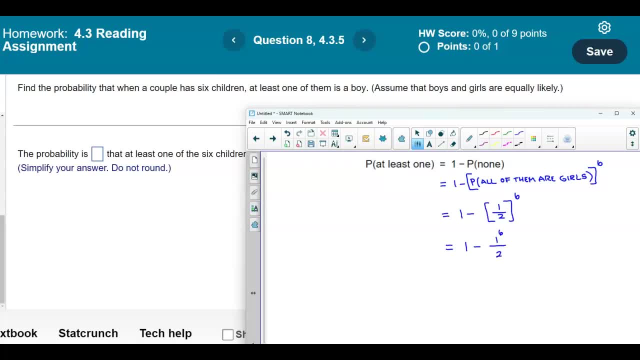 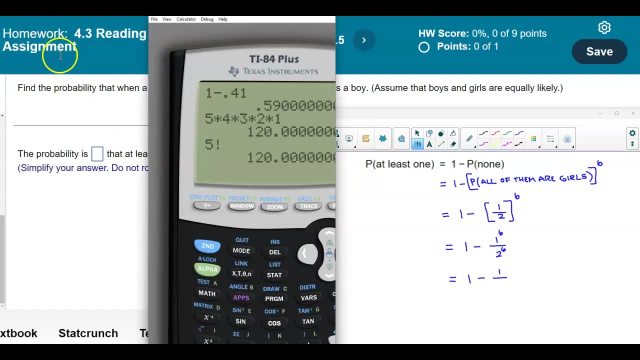 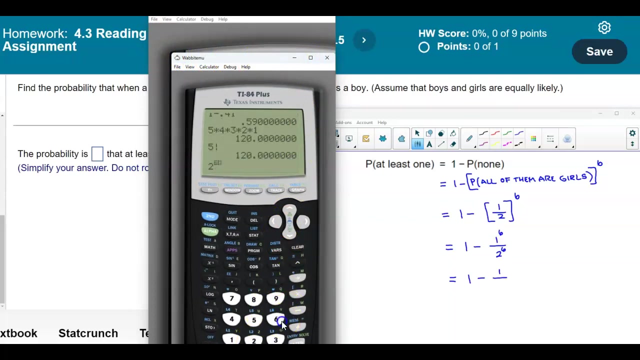 us one. So we have one to the sixth power and two to the sixth power. So that's going to give us one minus one. and then what is two to the sixth power? Well, we can go ahead and do that real quick on our calculator. So if we take two to the sixth, we're going to get 64.. Okay, so now they want us to put. 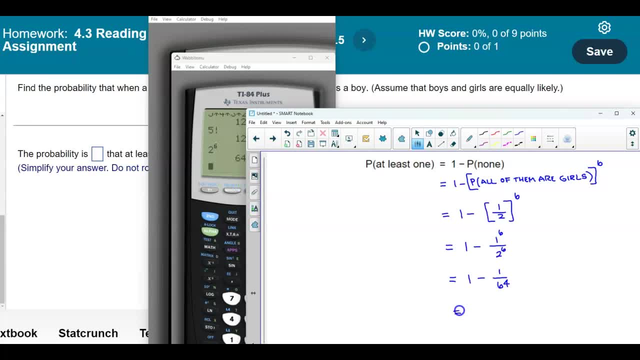 this in a fraction form, So remember that one is the same thing as 64 over two, So we're going to take 64 over 64.. So that's 64 over 64, minus one over 64, which is then equal to 63 over 64.. 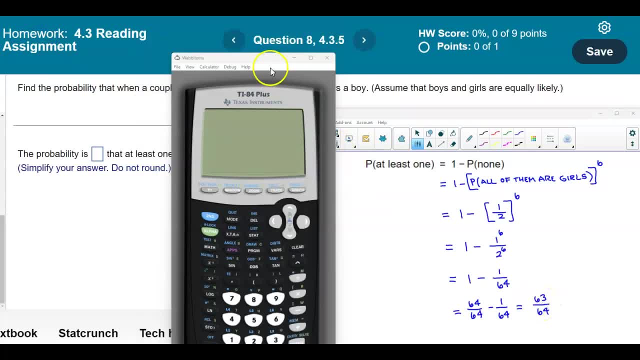 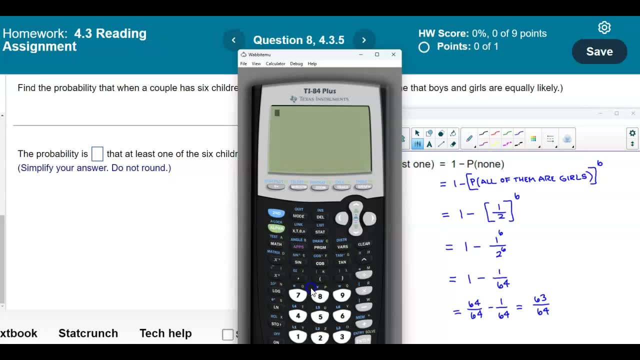 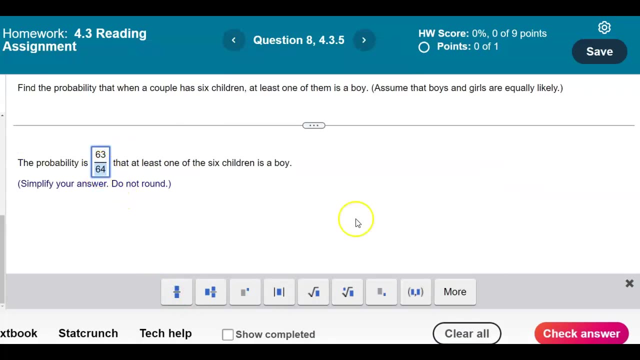 So we would have the probability of 63 or 64 over 64, and it says: to simplify the answer and do not round. So that means we're just going to put in the fraction of 63 over 64. so let's go ahead and put that in there- 63 over 64- and therefore there is our answer.